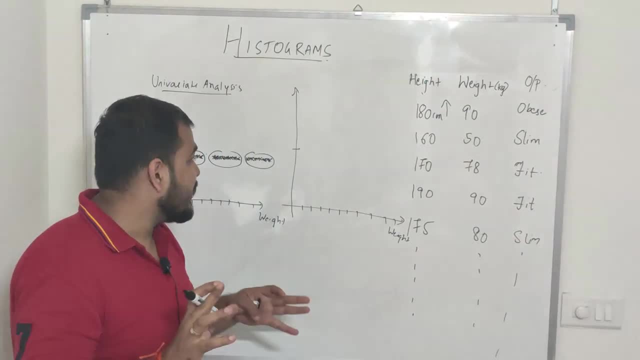 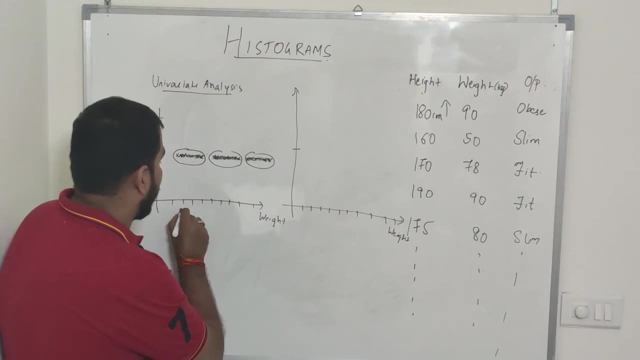 trying to understand how histogram is actually created. okay, and what exactly is histogram? Now? suppose in this particular range, suppose this particular range is between, just take as 80 to 90 kgs. Okay, now, in this particular range. you can see so many points are basically populated over there. 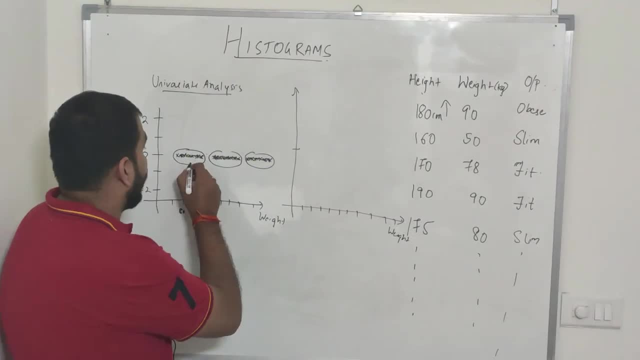 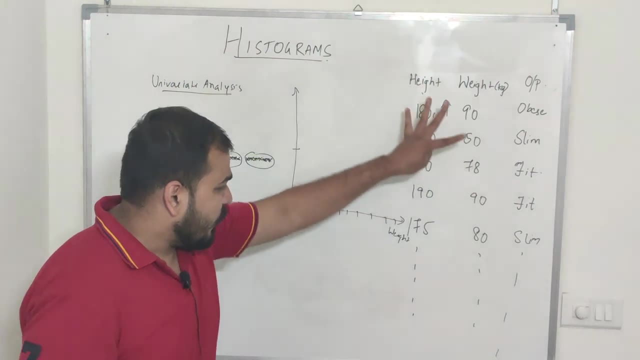 right and you don't know, like what will be the count, How many number of points are basically falling in this particular region, because there's so many points that are overridden over there. based on the data set that I Over here, I've just drawn a small data set. consider that I have. 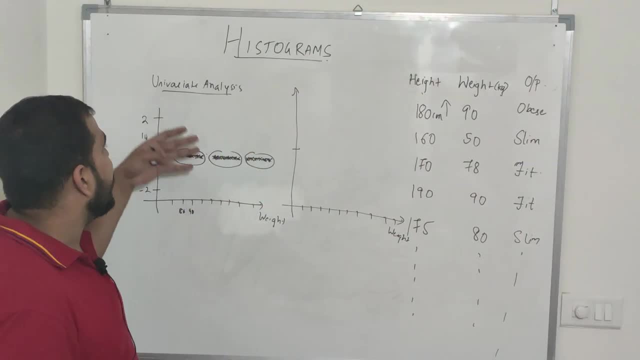 thousand records and I'm just trying to plot a 1D univariate analysis diagram. Okay, in the y-axis it will be zero, in the x-axis I'll be having the feature. Okay, so when I see this particular point, it's impossible for you to count, So histograms will help us to find out that within this particular 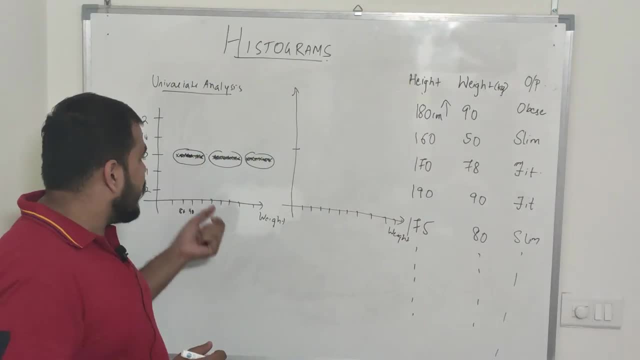 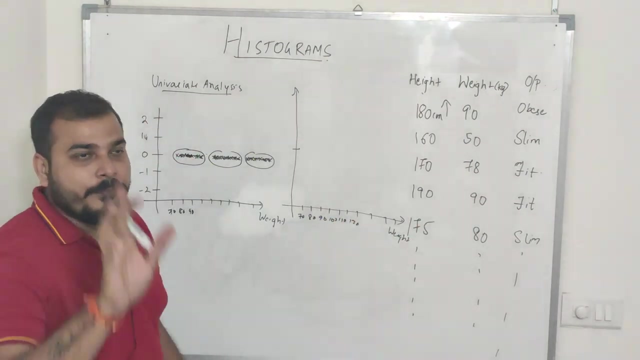 range. how many number of points are there right and based on that, a building will be created. a bar graph will basically be created. Suppose between 70 to 80, suppose. consider this is my 70, 80, 90, 100, 110, 120 and like this, all the values are there. Consider that within 70 to 80, they are around 10. 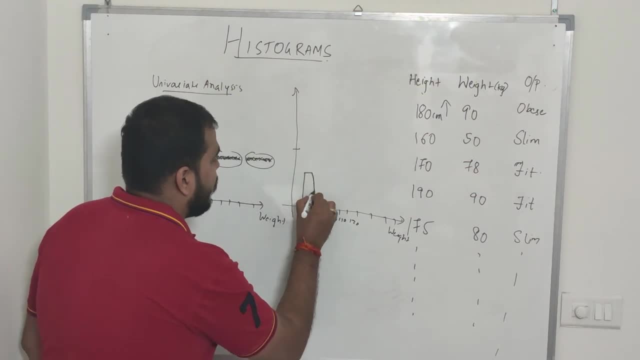 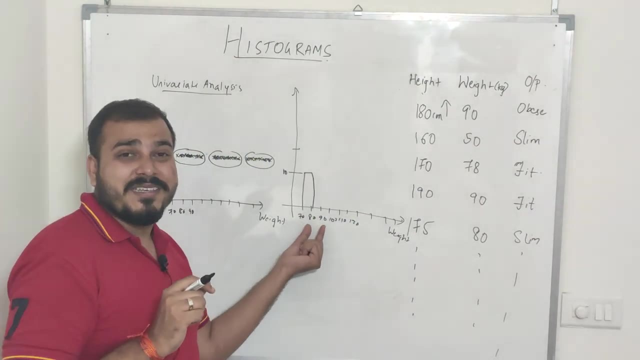 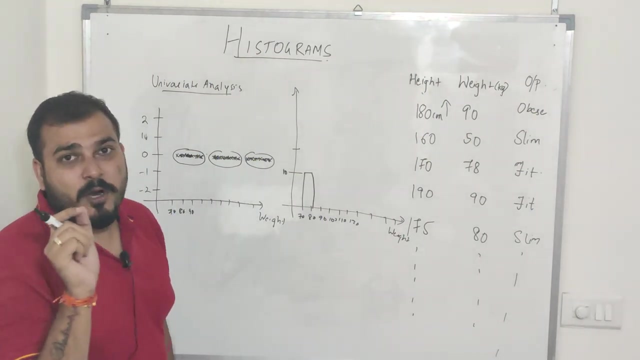 number of points. Okay, So in this a plot will get created with the help of histograms and this value will basically be 10.. This is basically indicated, indicating that within the bin range between 70 to 80, 10 count 10 values are basically present. Similarly, between 80 to 90. I see more dense points are there, So I can. 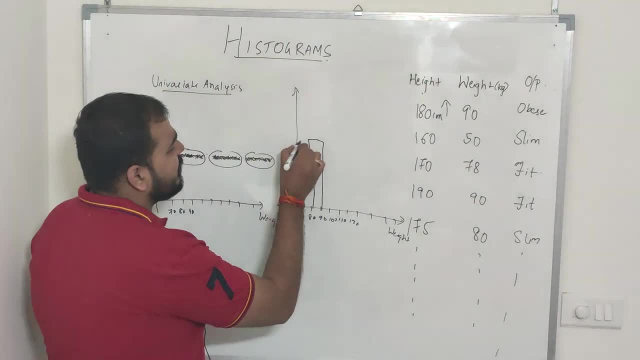 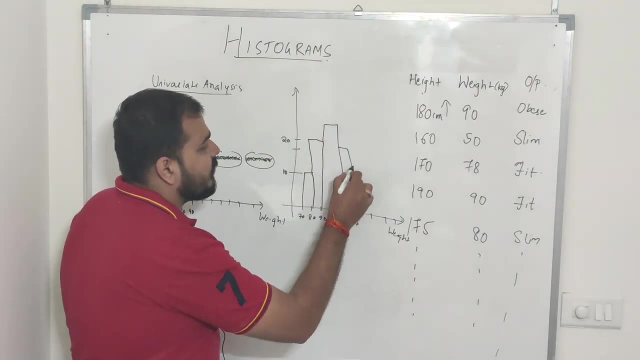 basically think that, okay, this may be 20.. Okay, this. this is basically showing us that what is the count? Okay, and like this, all the graphs will be created. Okay, all the graphs will be created. you will be able to see this particular graph. Okay. 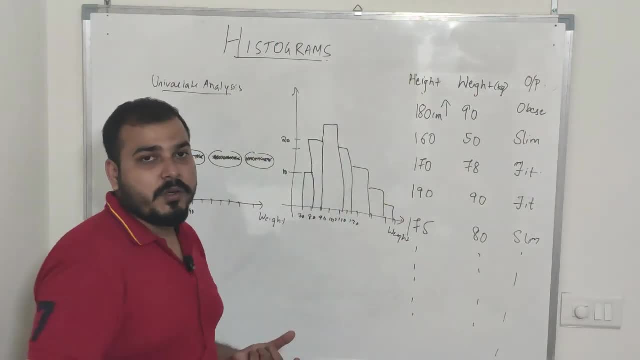 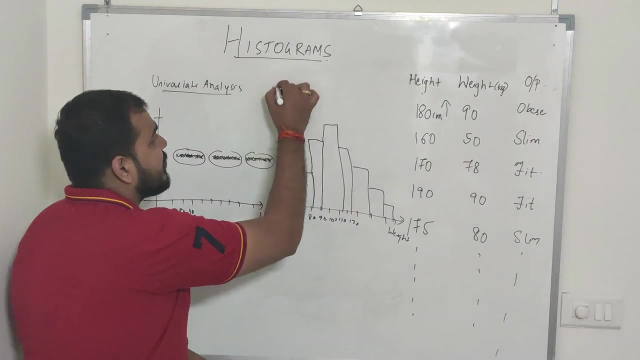 Okay, Just like this, and that is what is basically histogram. you know, a histogram helps us to find out that how many points has been populated in the left hand side, that is, in my y-axis. is basically shows us the count count of the number of values that are present within this. 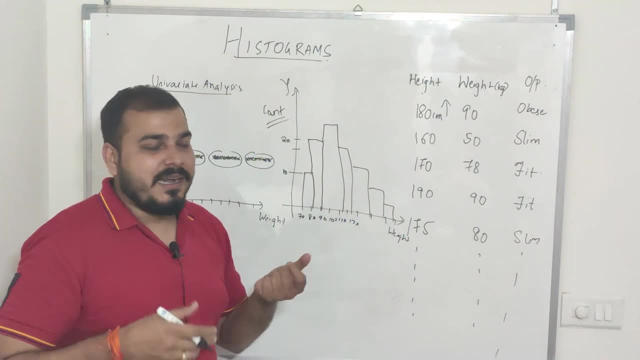 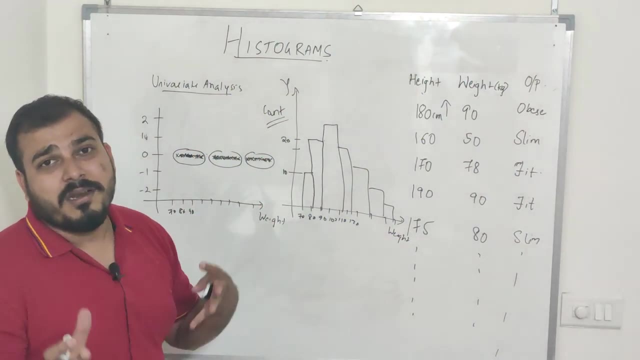 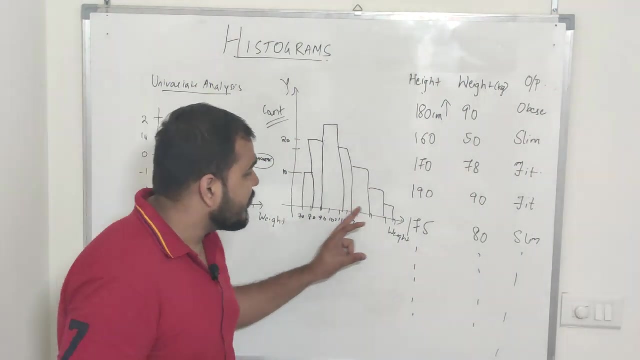 range and based on that this building is basically created. right, and it is very, very easy to plot histogram. you can use matplotlib hist function or you can also use seaborn- there is an- again a histogram function for that Okay- Where you can basically plot it and always remember guys whenever you are plotting this. 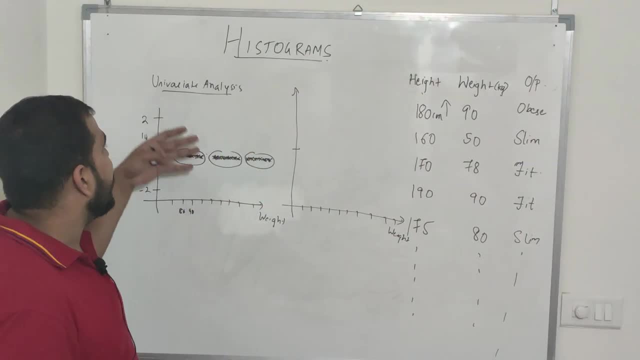 thousand records and I'm just trying to plot a 1D univariate analysis diagram. Okay, in the y-axis it will be zero, in the x-axis I'll be having the feature. Okay, so when I see this particular point, it's impossible for you to count, So histograms will help us to find out that within this particular 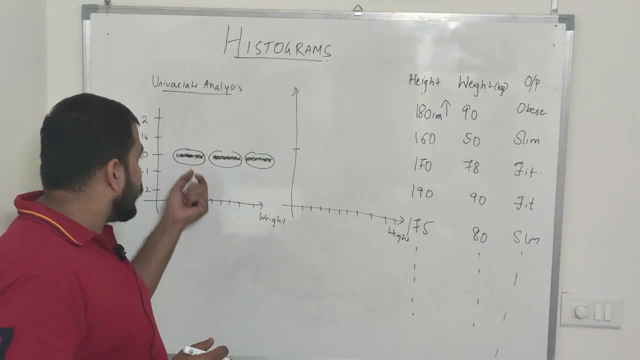 range. how many number of points are there right and based on that, a building will be created. a bar graph will basically be created. Suppose between 70 to 80, suppose. consider this is my 70,, 80,, 90,, 100,, 110, 120 and like this, all the values are there. Consider that within 70 to 80 they are. 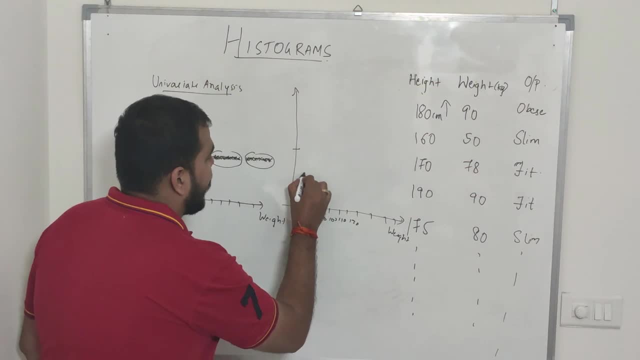 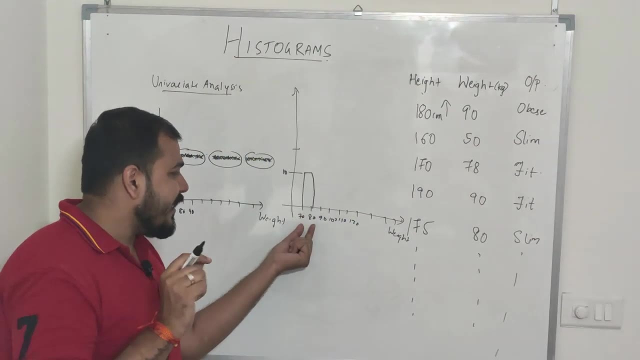 around 10 number of points. Okay, A plot will get created with the help of histograms and this value will basically be 10.. This is basically indicated, indicating that within the bin range between 70 to 80, 10 count 10 values are: 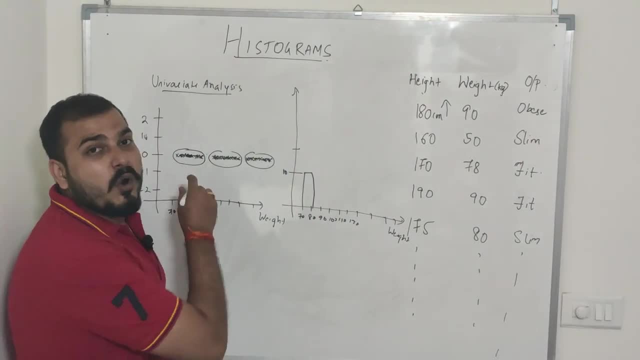 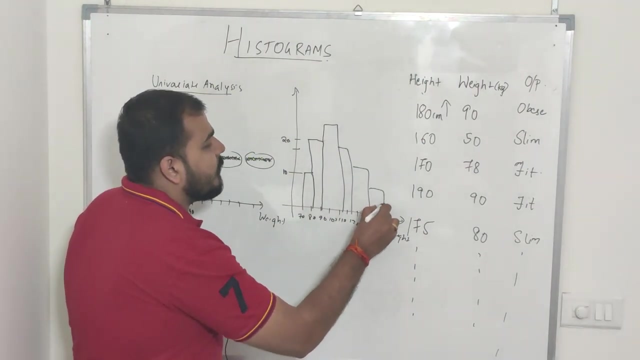 basically present. Similarly, between 80 to 90. I see more dense points are there, so I can basically think that, okay, this may be 20.. Okay, this, this is basically showing us that what is the count? Okay, and like this, all the graphs will be created. Okay, all the graphs will be created. you will be able to. 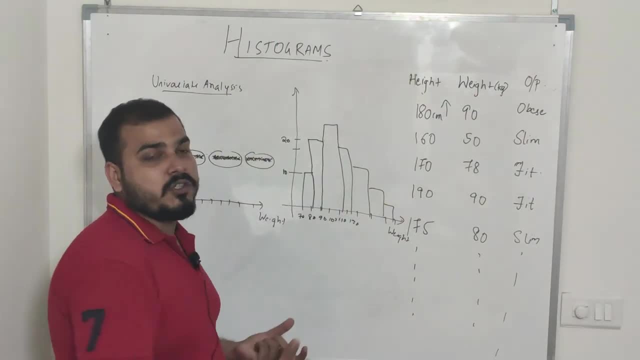 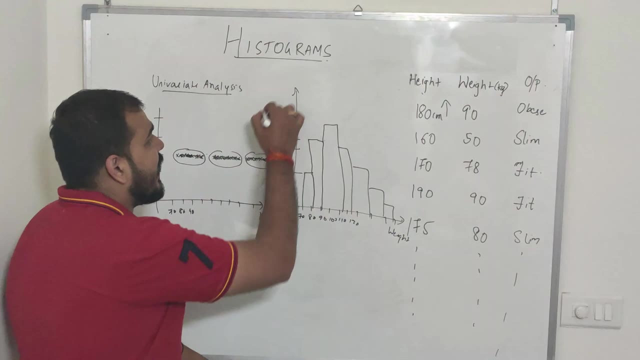 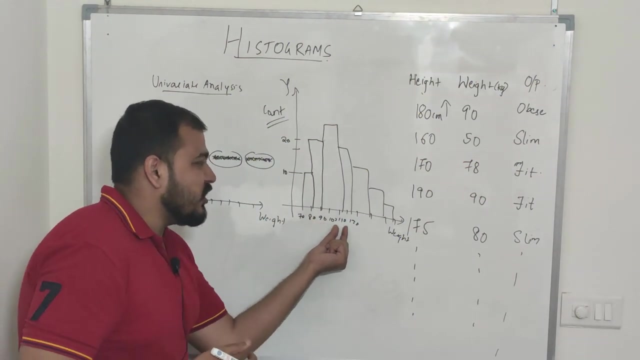 see this particular graph. Okay, Like this, and that is what is basically histogram. you know, a histogram helps us to find out that how many points has been populated in the left hand side, that is, in my y-axis. is basically shows us the count count of the number of values that are present within this range and, based on that, this, 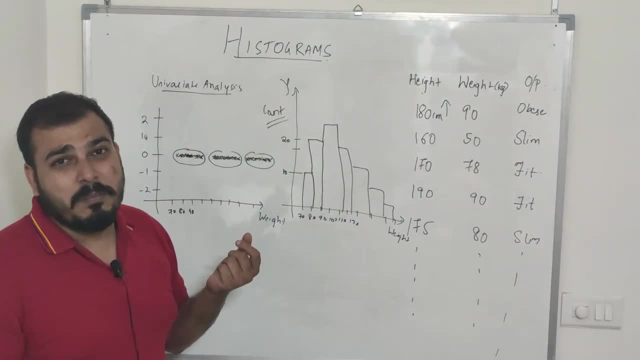 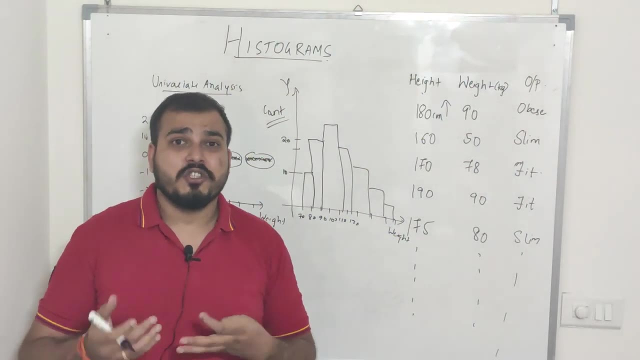 building is basically created right, and it is very, very easy to plot histogram. you can use matplotlib hist function or you can also use seaborn. there is an again a histogram function for that, where you can basically plot it and always remember, guys, whenever you are plotting this histogram it. 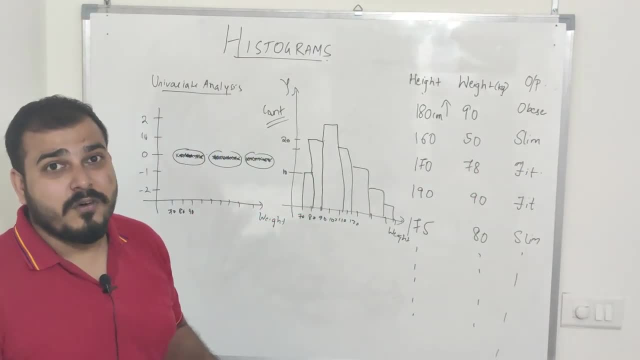 will be with respect to one feature. yes, you can combine three to four features and based on- uh and again, not just like this- multiple diagrams you basically have to create. but this is making you understand, and this is also important, guys, because, if you see this, when I try to create a figure like